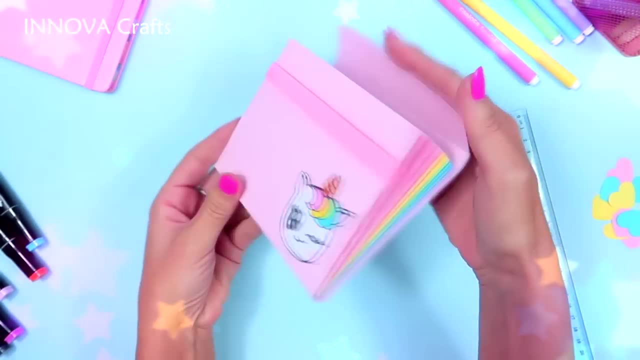 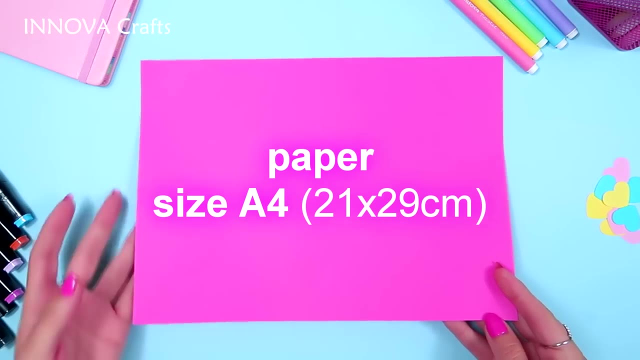 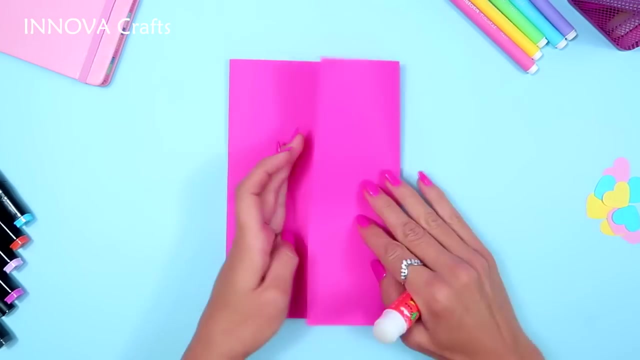 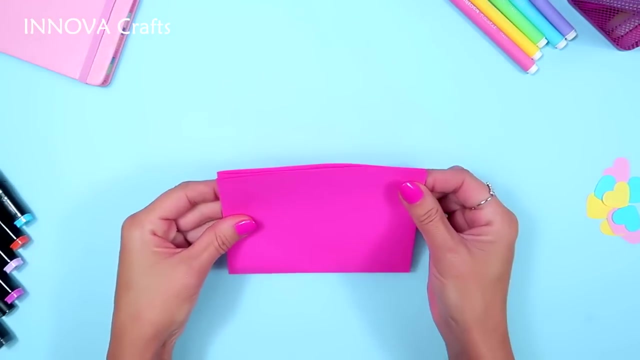 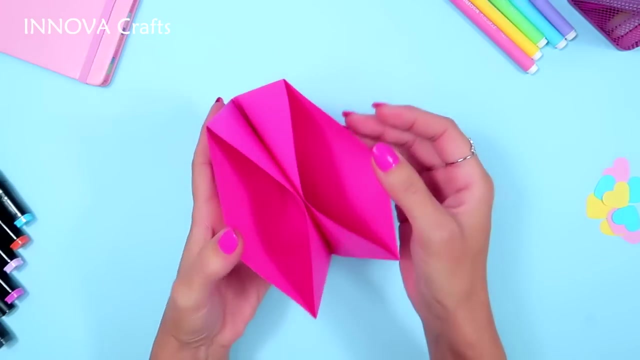 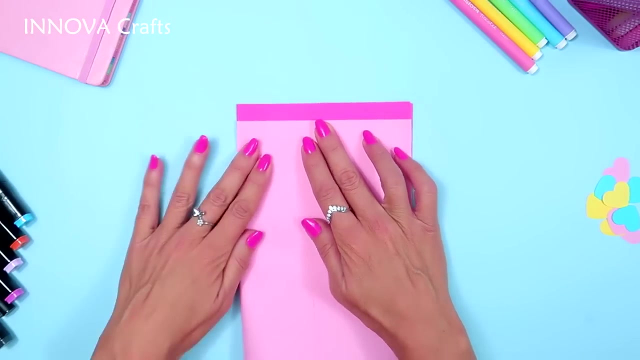 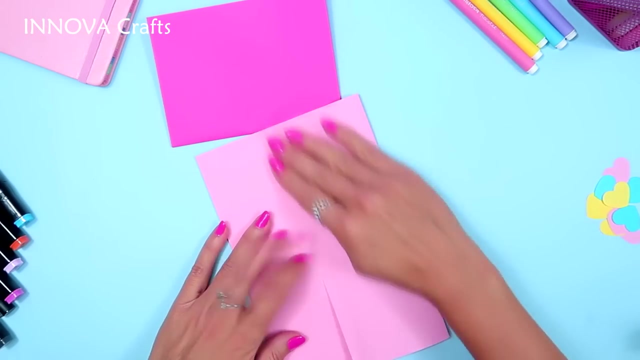 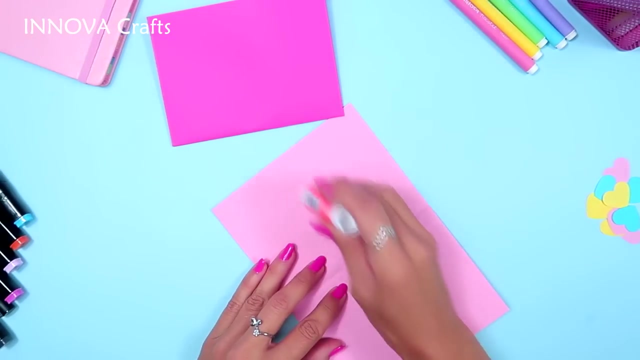 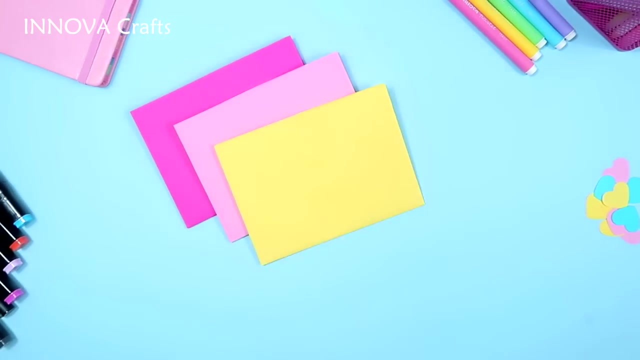 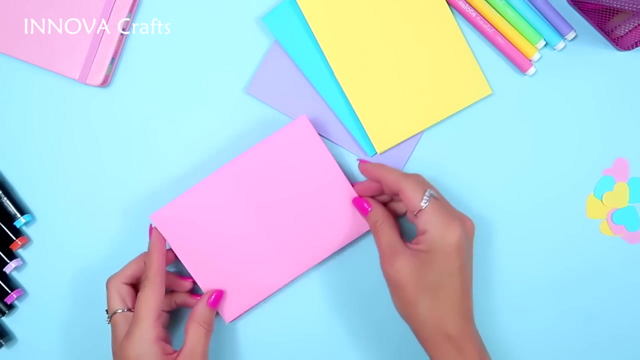 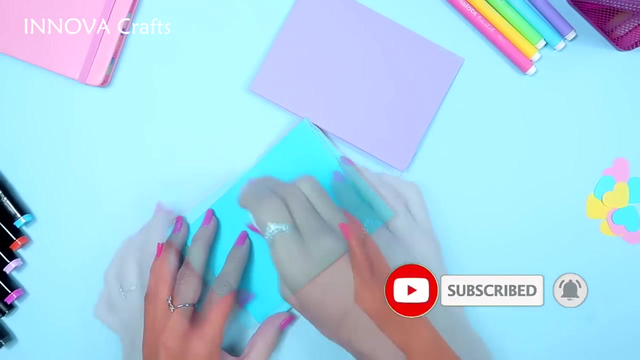 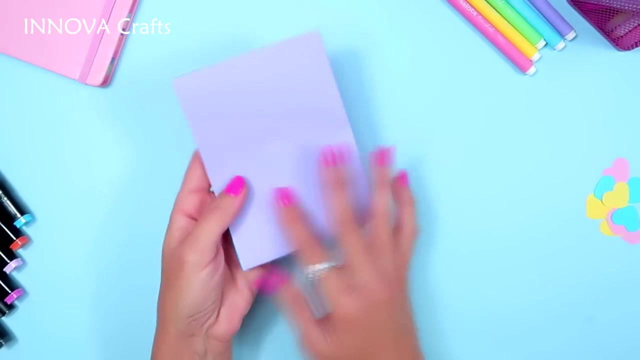 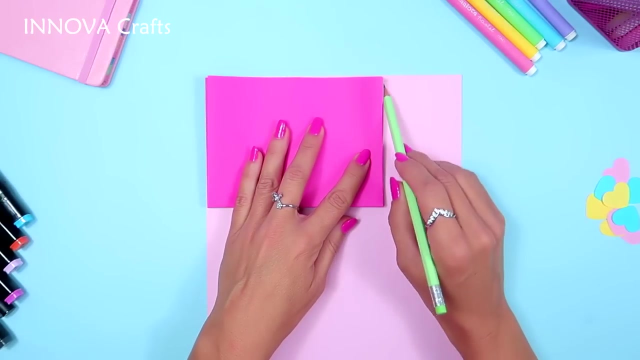 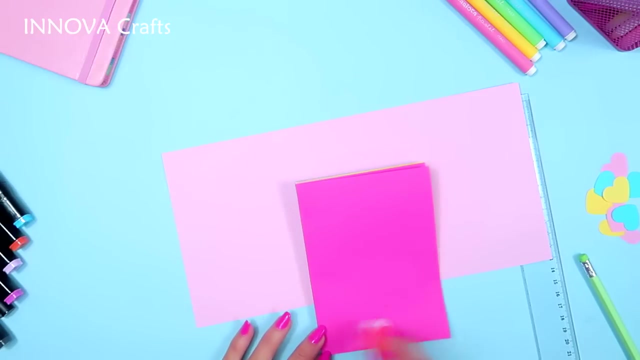 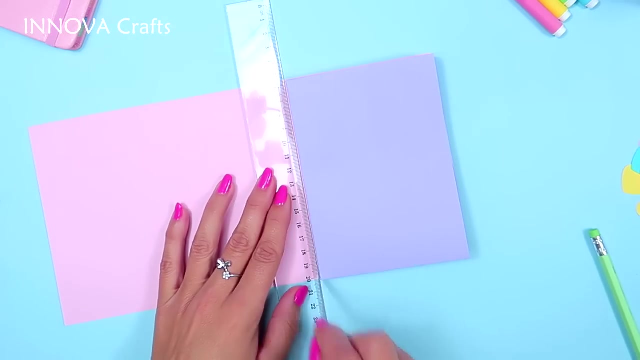 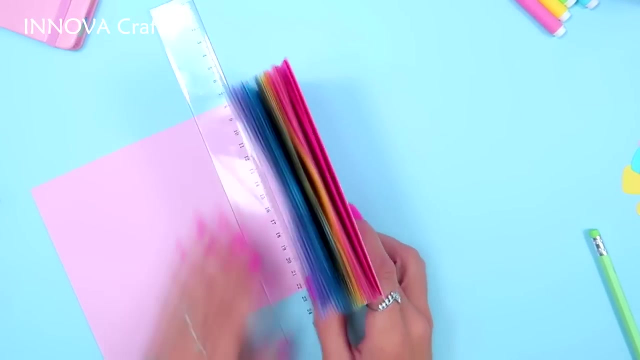 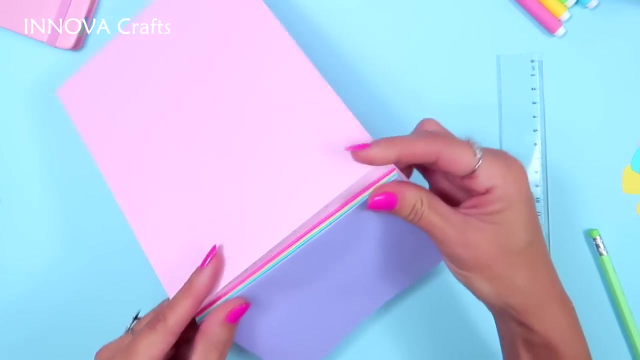 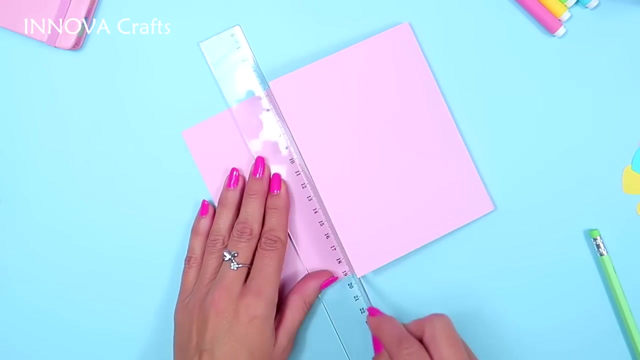 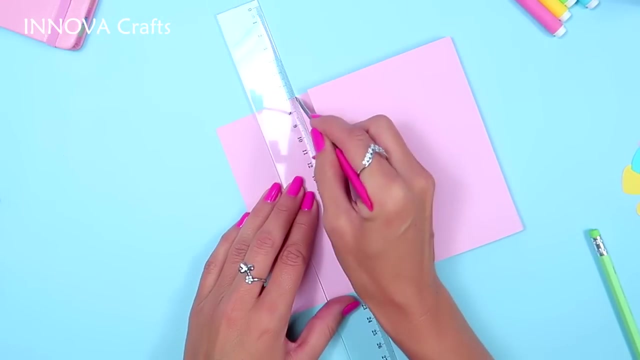 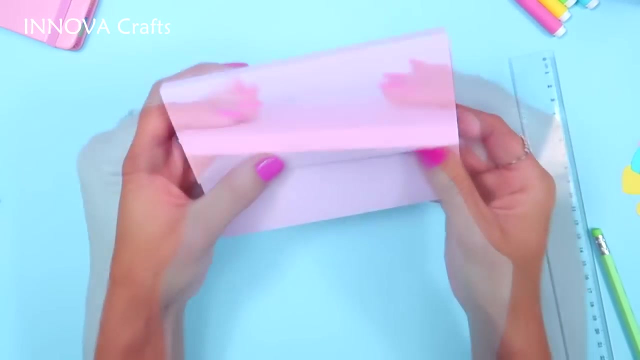 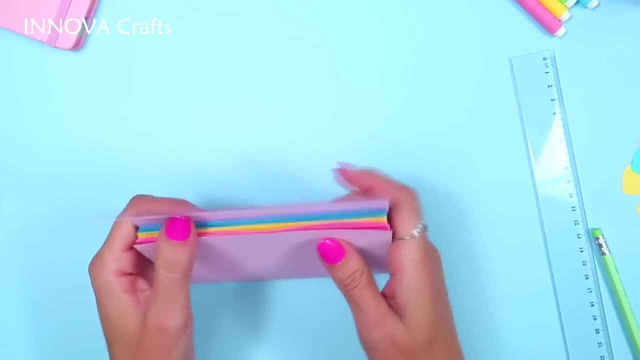 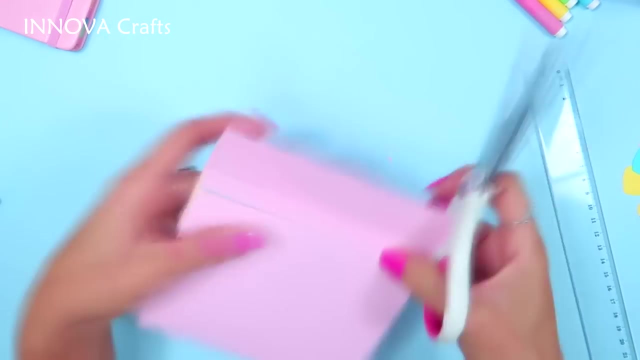 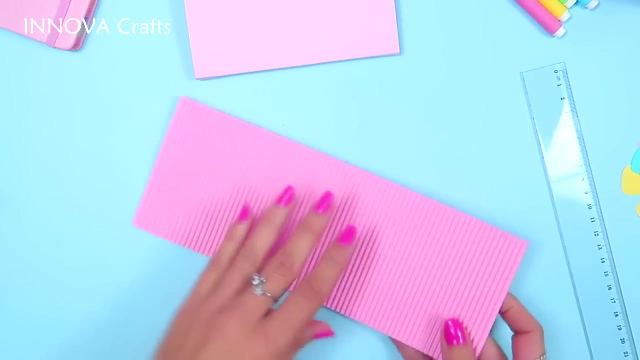 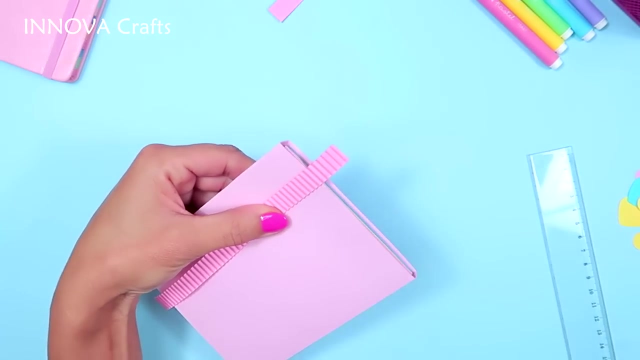 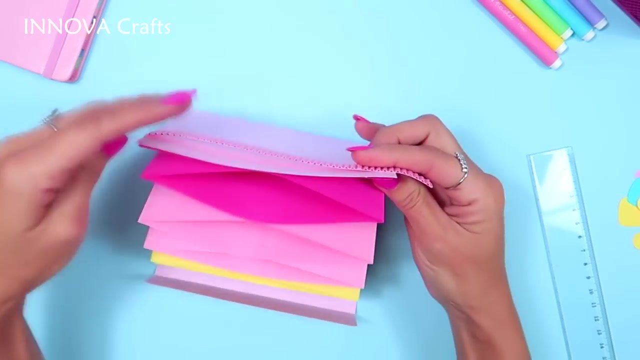 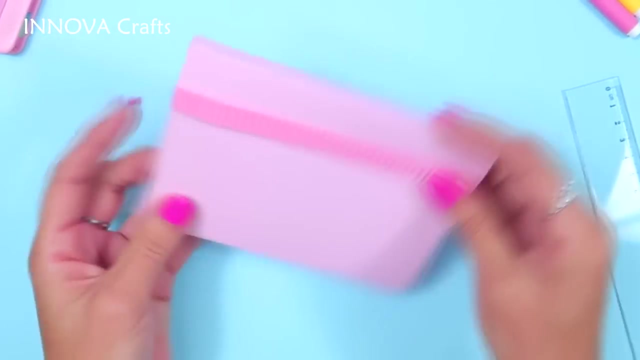 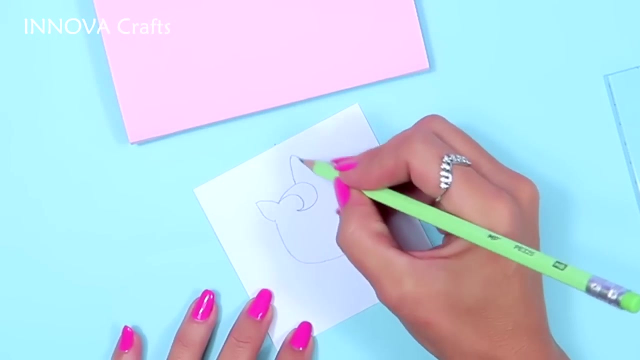 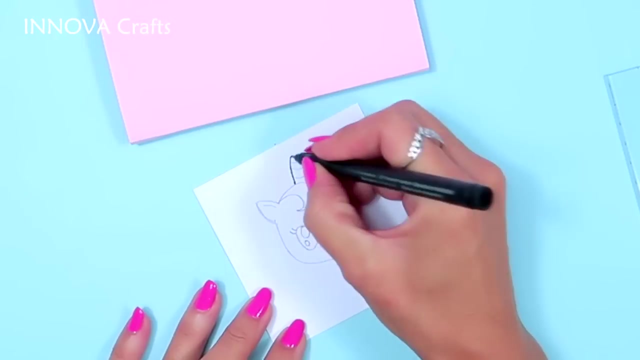 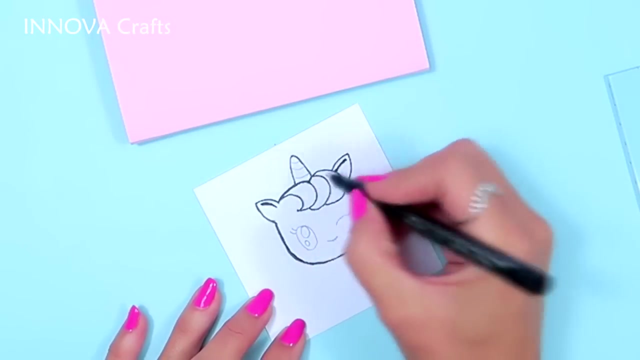 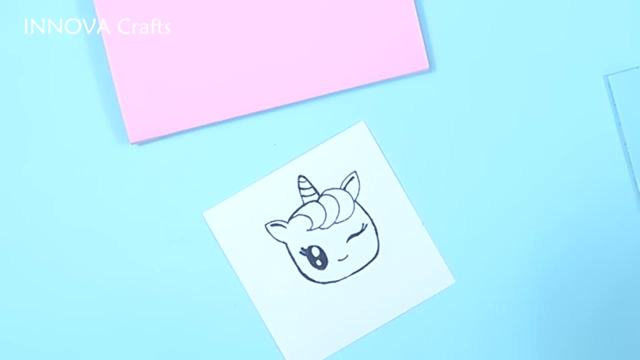 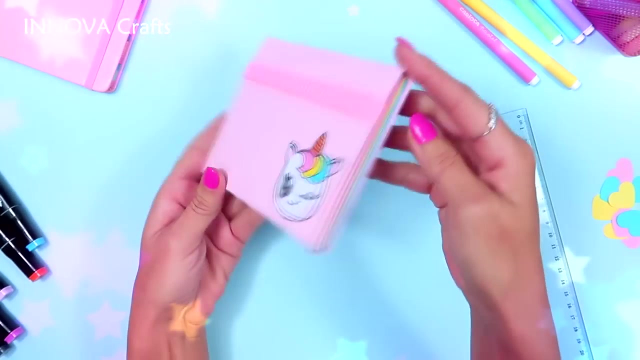 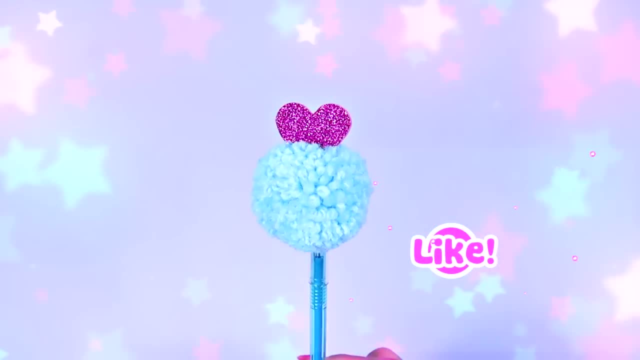 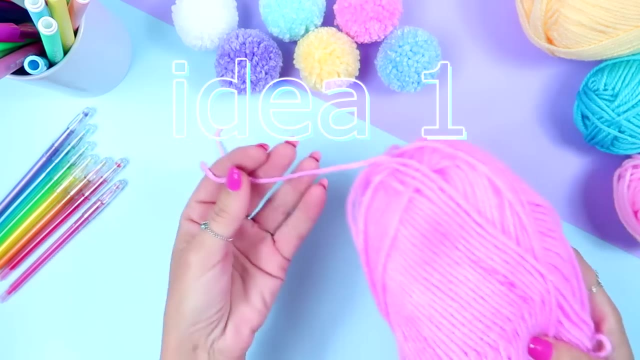 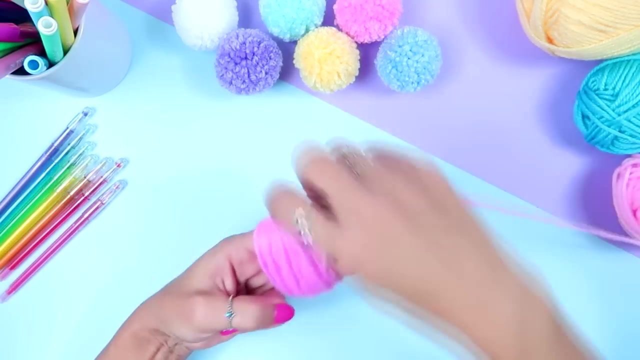 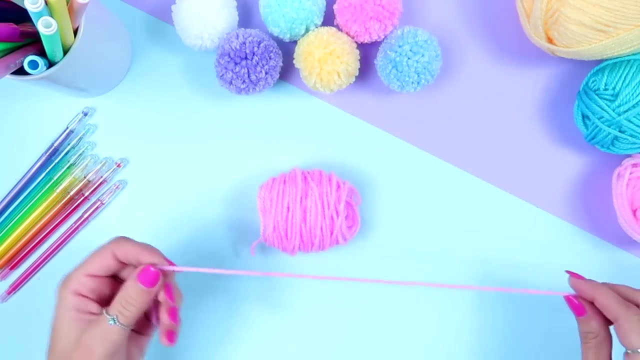 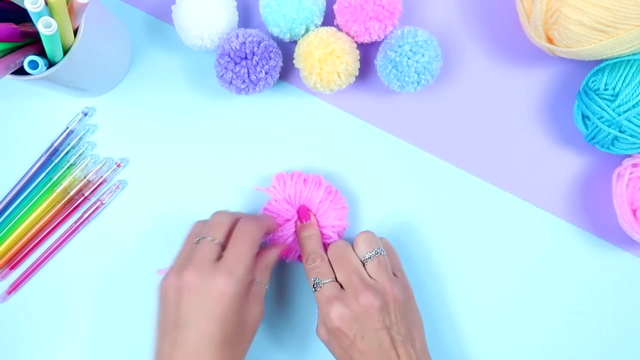 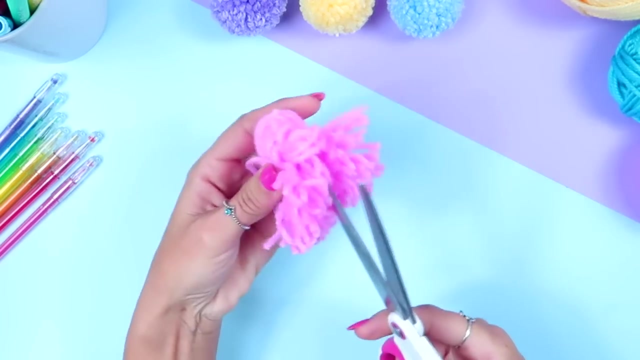 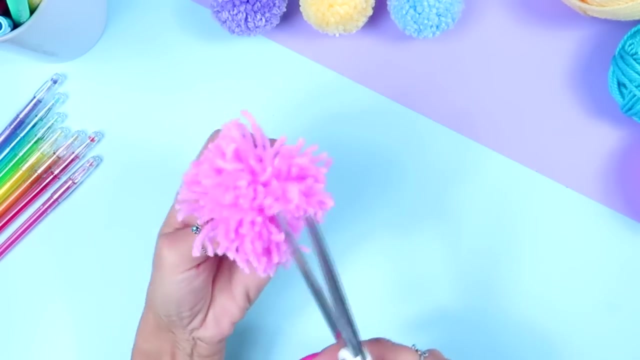 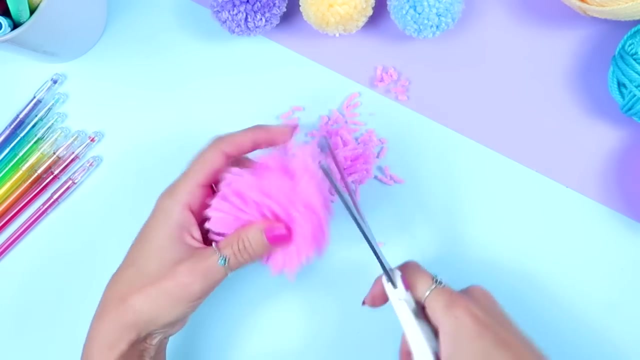 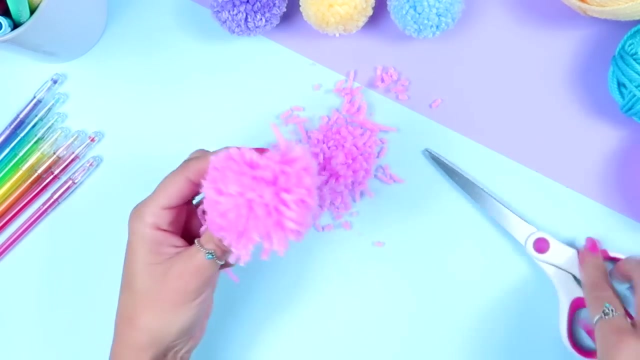 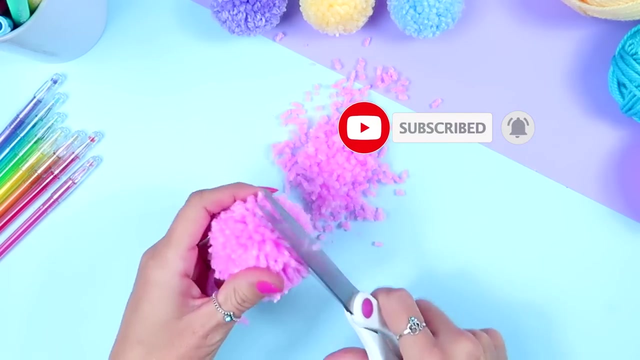 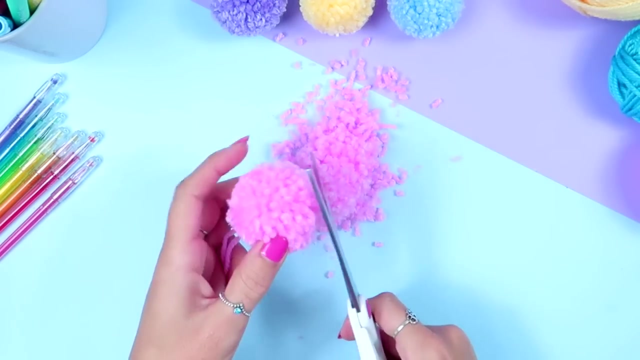 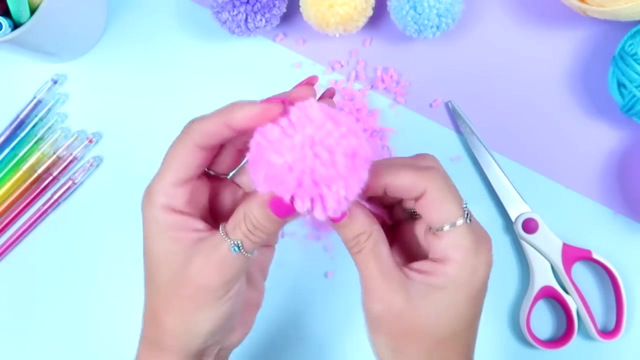 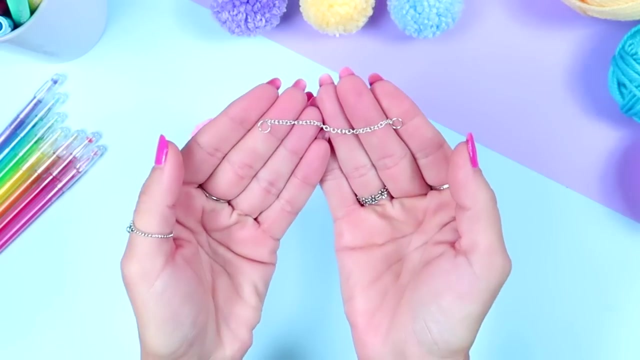 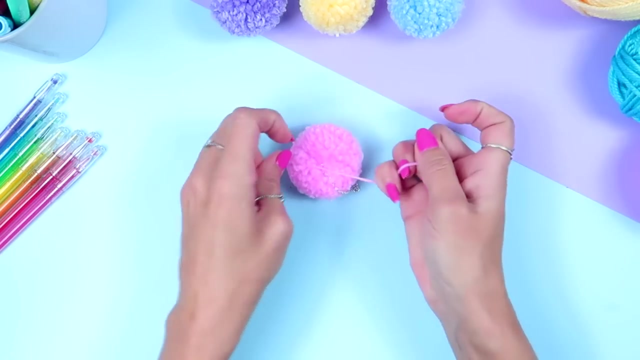 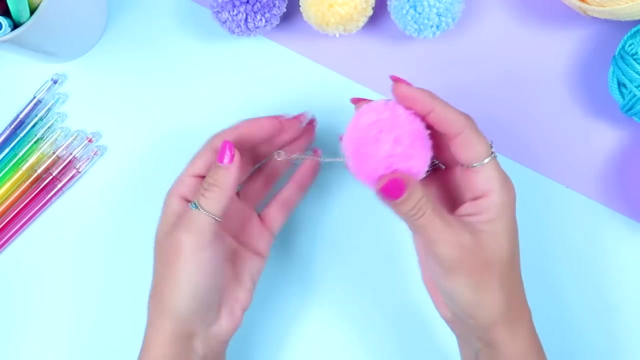 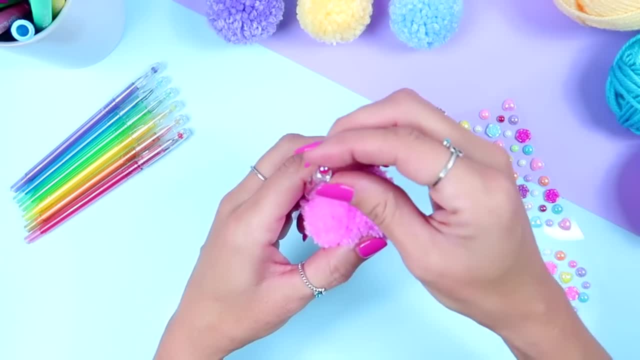 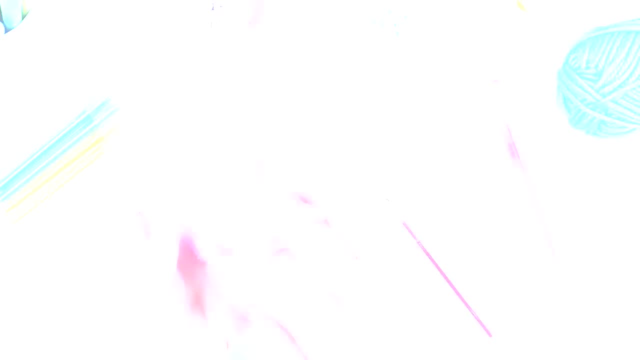 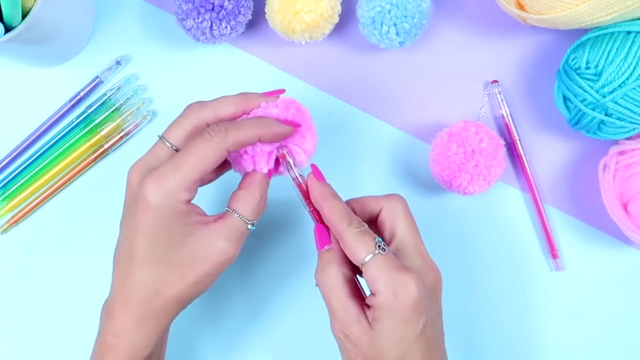 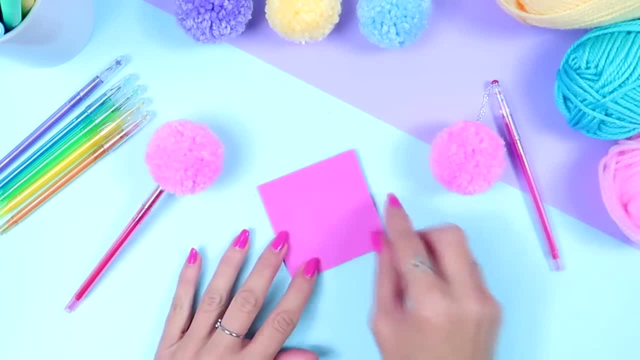 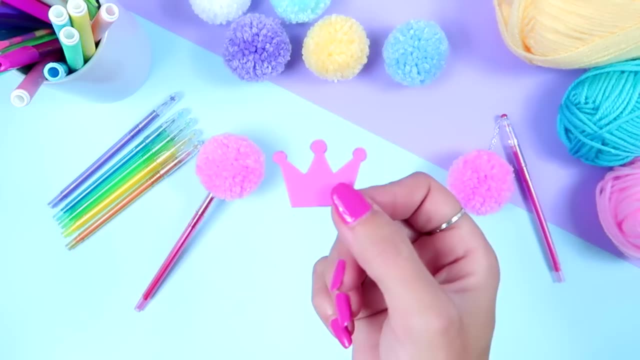 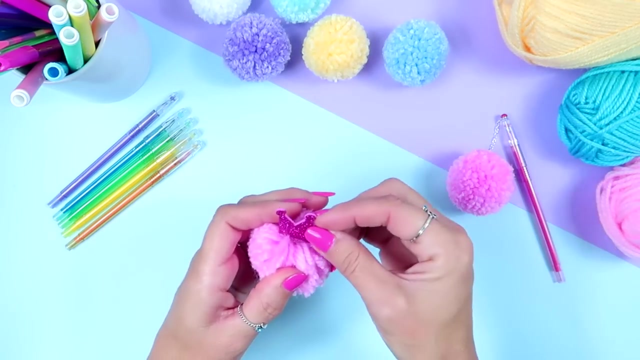 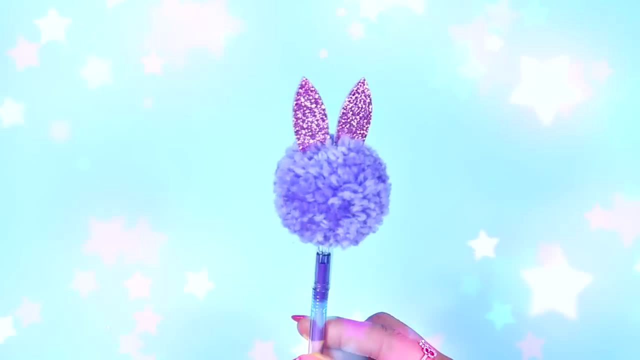 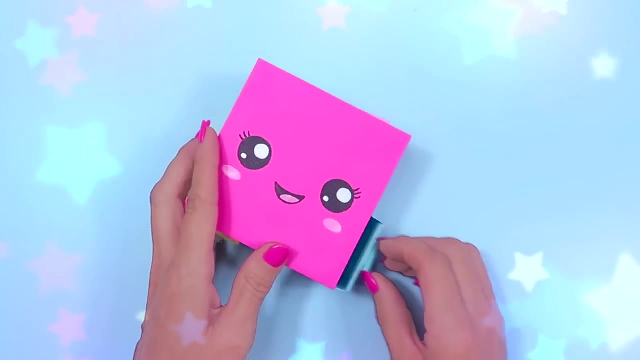 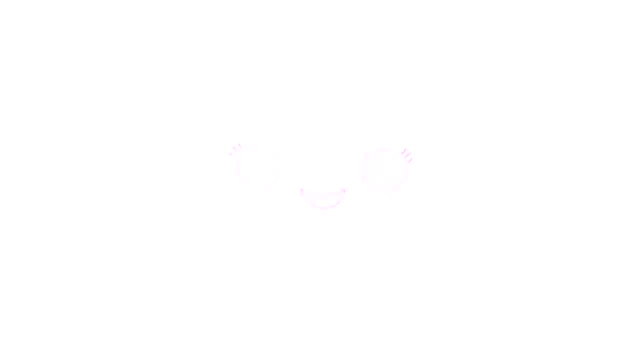 Love how you make me feel alive When you're with me. If you need a hand, I am here for you. If you could ask, I'll lead you back up. Walk that extra mile. I would do that too, Just so I could be beside you. 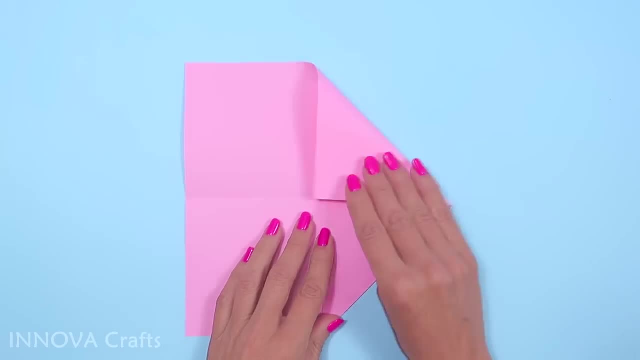 If the end is near, just know that I got you. I'm your armor when things get tough. Now I got you back. your battle's a mine too. I'll fight for you when things get hard. Lay it all on me When you're with me. 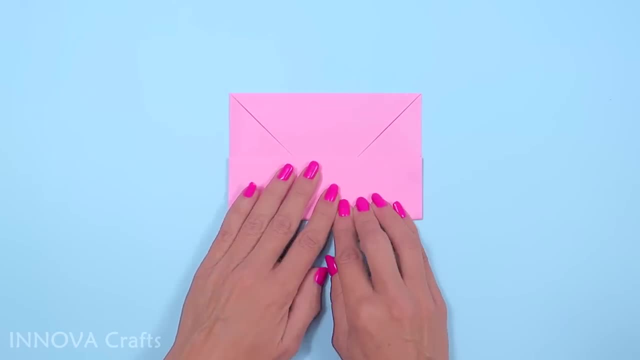 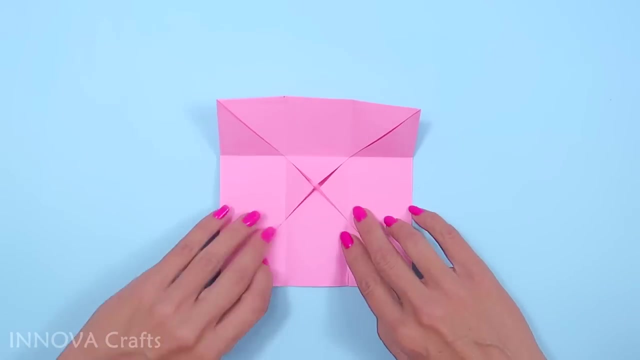 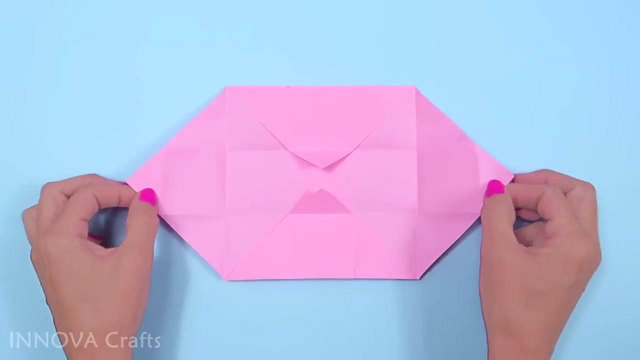 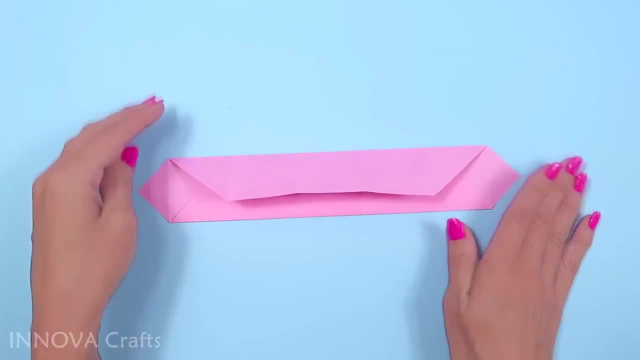 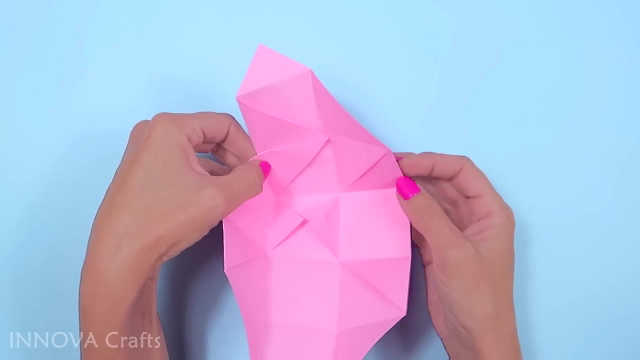 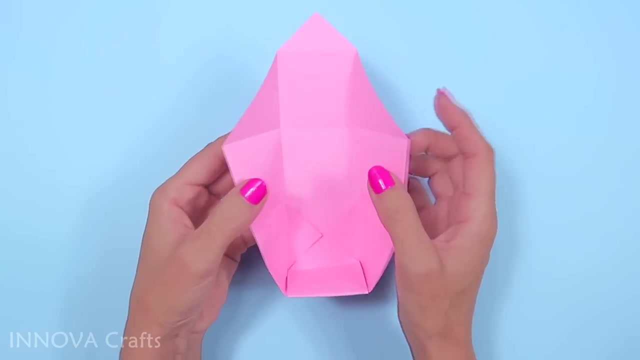 I know the world can be a crazy place sometimes, But now that I am here beside you, We can leave tonight. leave it all behind. Instead of a song: brand new Baby. you should know I got you. If the end is near, just know that I got you. 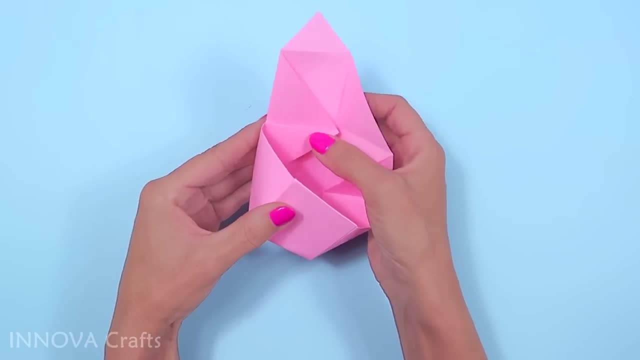 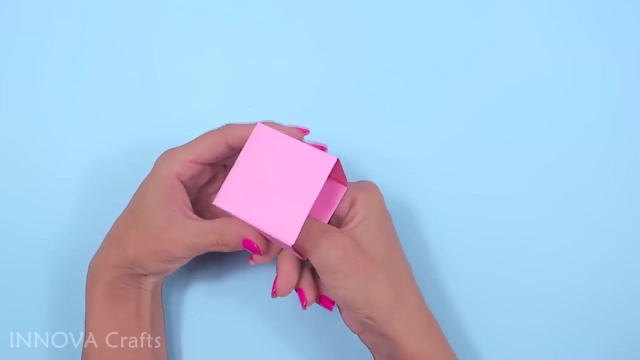 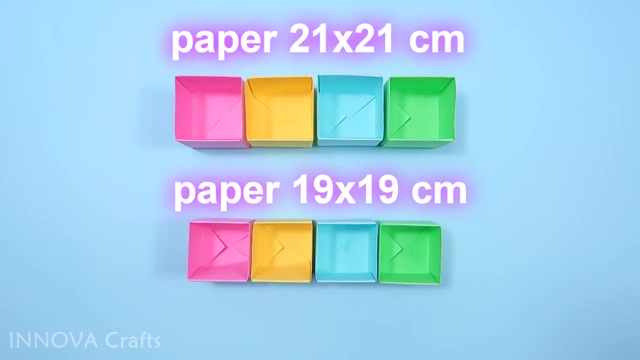 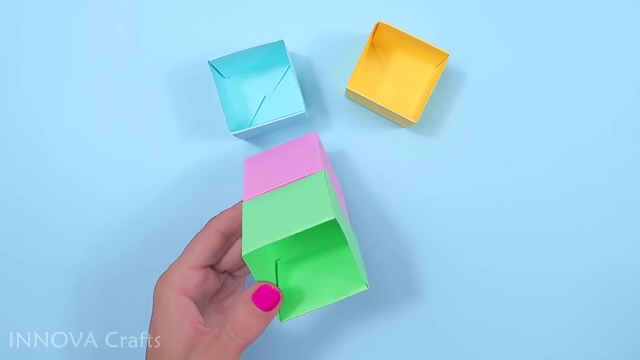 I'm your armor when things get tough. No one got you back. your battles are mine too. I'll fight for you. when things get hard, Lay it all on me. When you're not strong enough to carry on, Baby, you should know I got you. Baby, you should know, I got you. 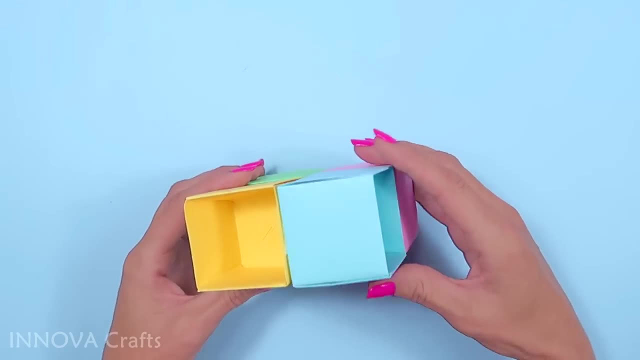 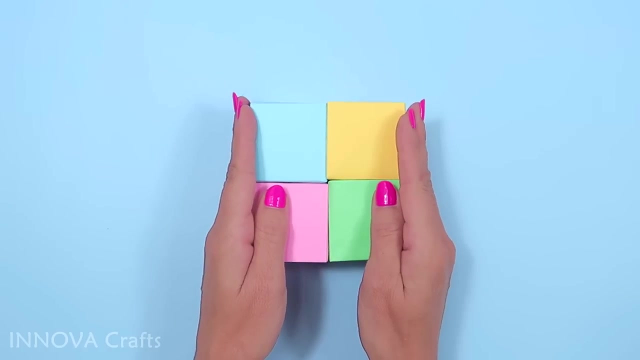 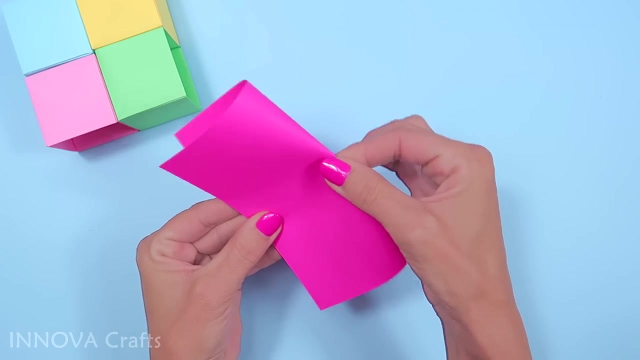 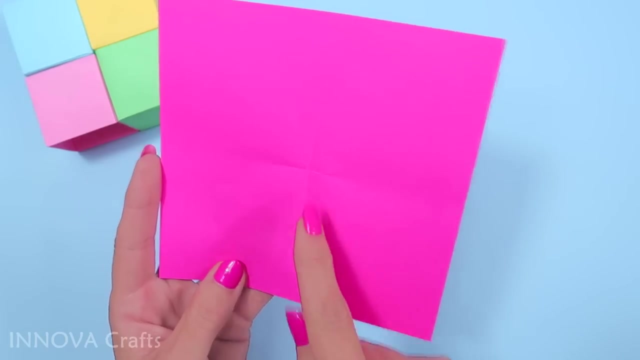 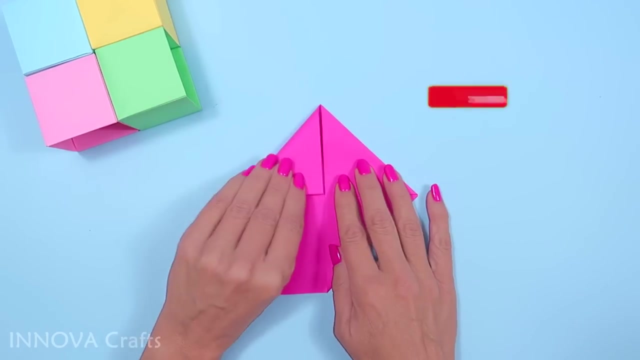 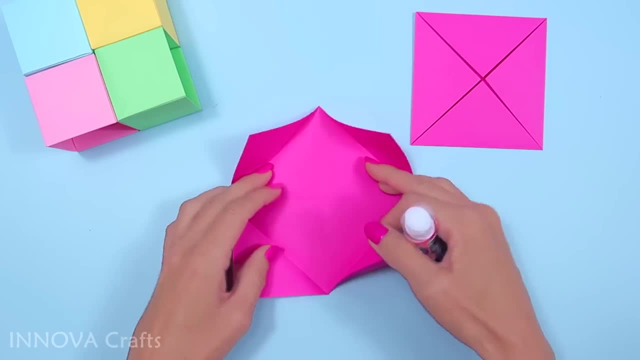 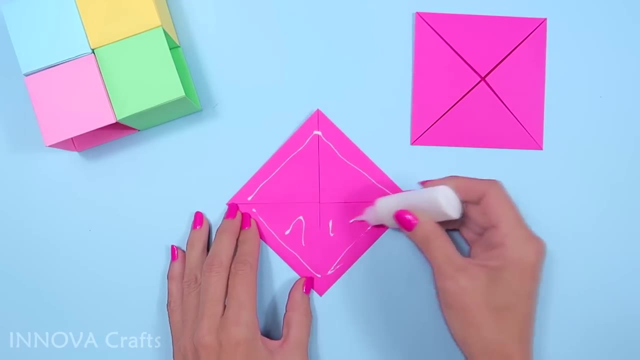 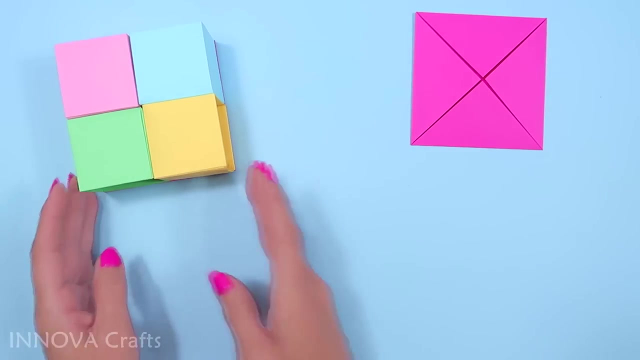 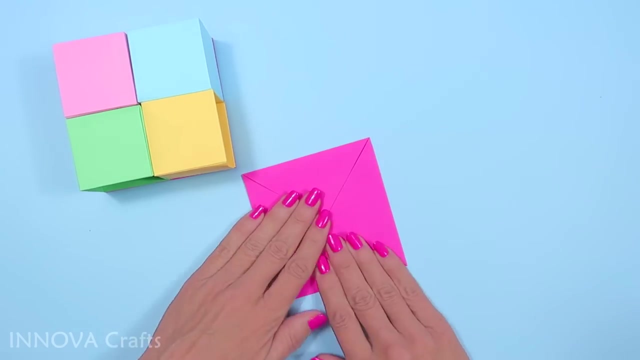 You say all the right things. when I'm hurting, You always pick me up. when I am down, It's like you have a spark that leaves me burning. You just have your ways to get me high. You make all my dreams come true. It feels right when I'm around you. 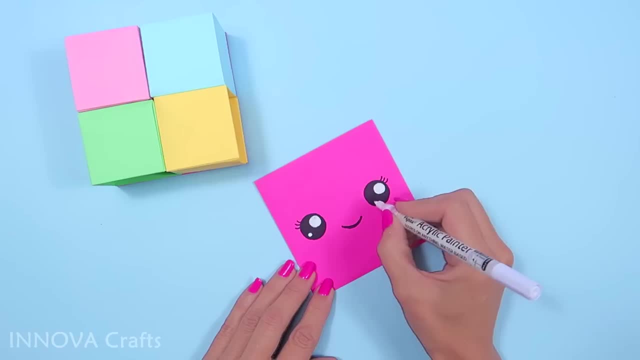 We could break up and then make up. I always come back to you. You move me in a way never thought anyone could You give me high. you're my drug. When I am feeling down, I'm feeling down. You make all my dreams come true When I am feeling blue. 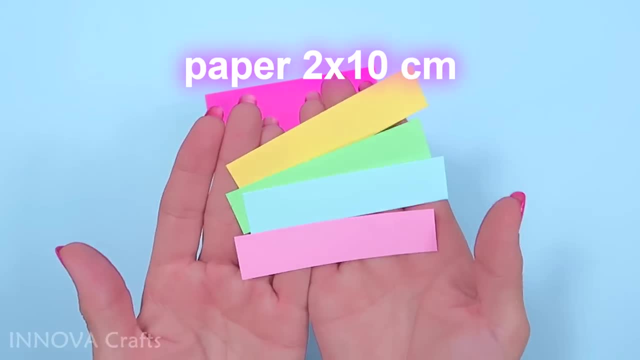 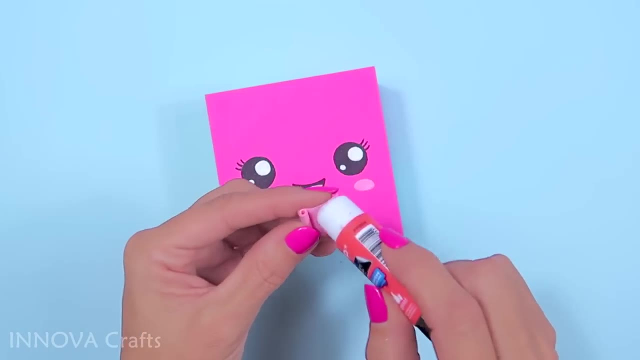 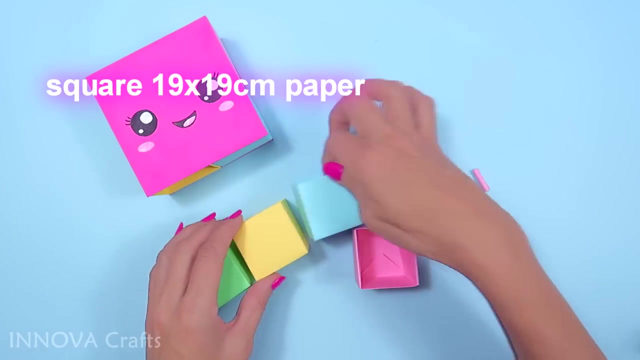 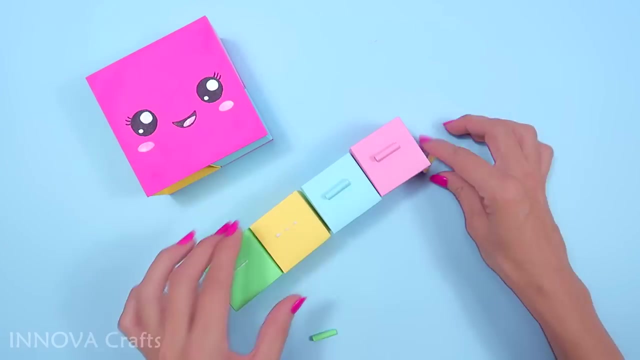 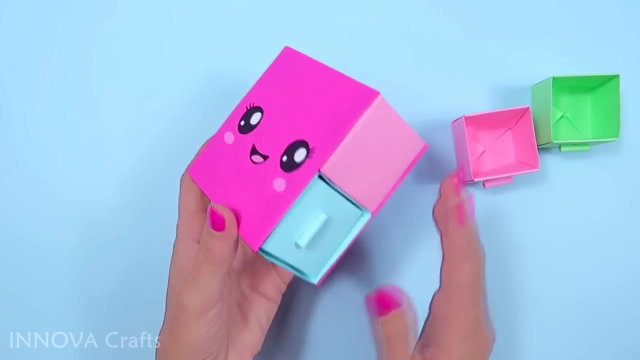 Yeah, it's all you Cause. you're the one, Yeah, the one, Yeah, you're the one, Yeah the one. You touch me in a way that makes me shiver. Sometimes I can't believe that you are mine. Love's a gun and baby, you're my trigger. 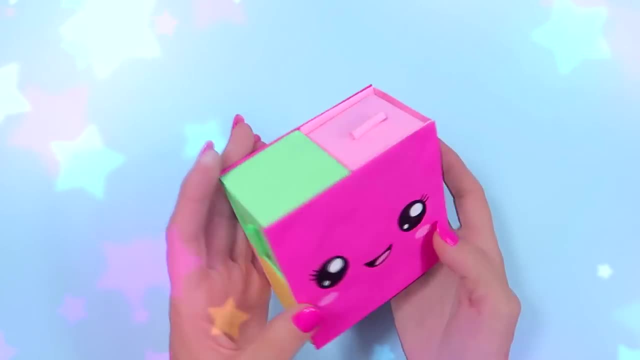 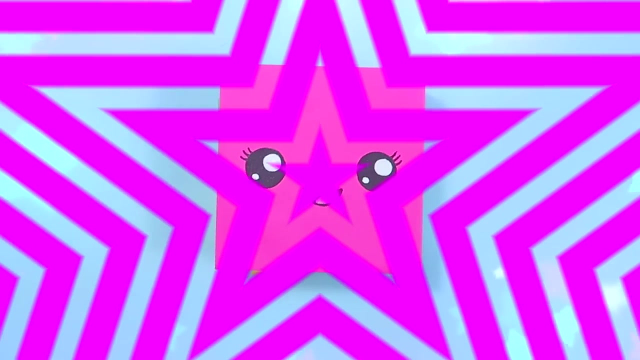 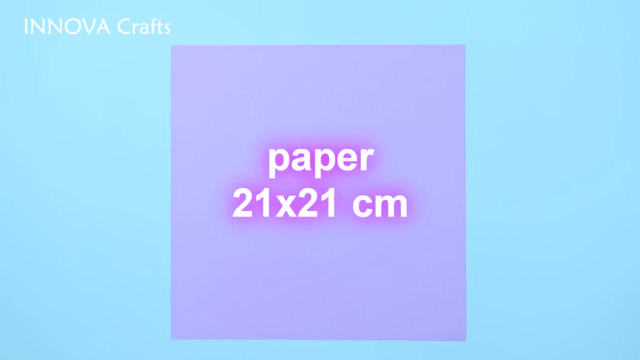 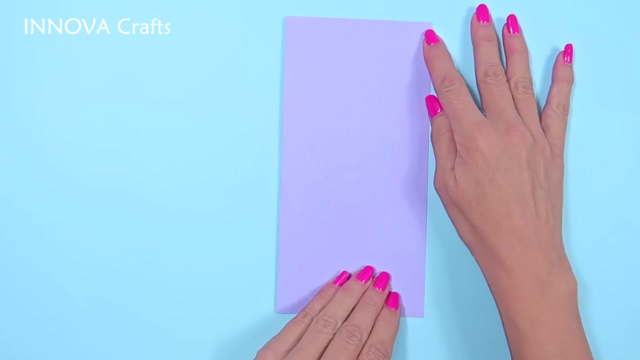 You kiss me in a way that gets me high. You make all my dreams come true. It feels right when I'm around you. I get so caught up in the middle, Thinking of drowning in those blue eyes. I'm losing sight cause I am falling. I'm so deep down, deep down. 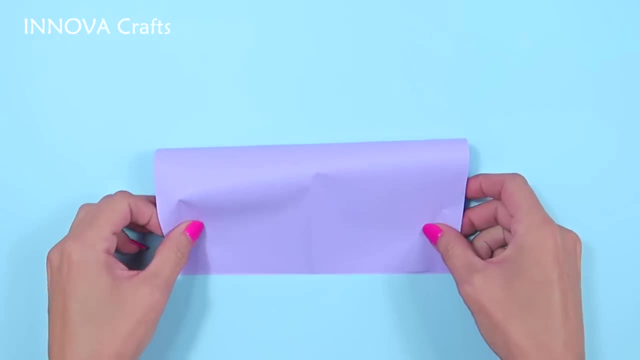 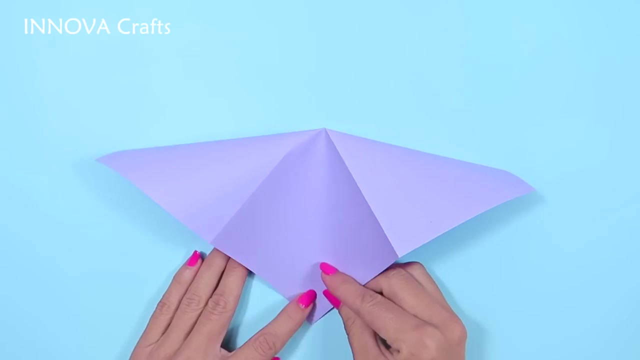 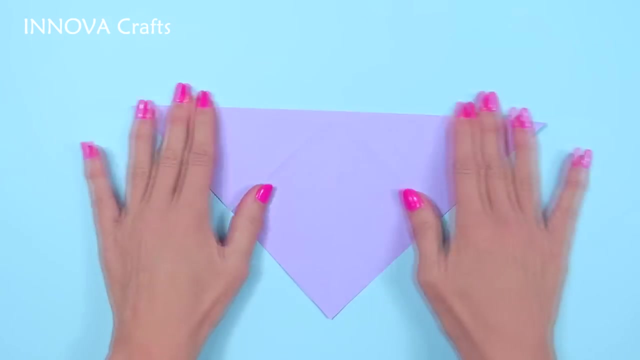 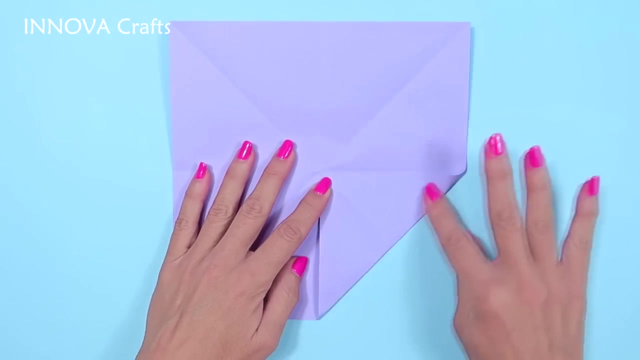 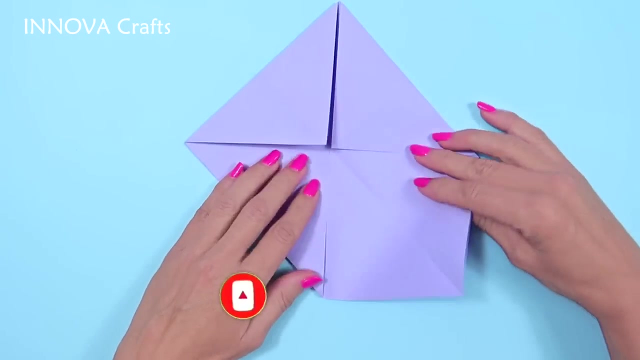 And it's not a lie That I die. I can't hide What this is. Yeah, I keep drowning in those blue eyes And you can tell me all the fair lies. I will put out all of the fire If it gets too dark. I'll be your light. 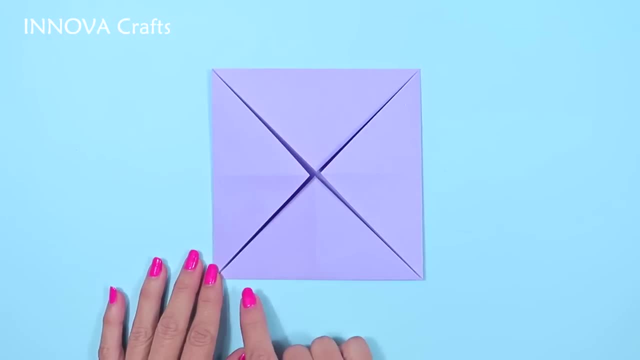 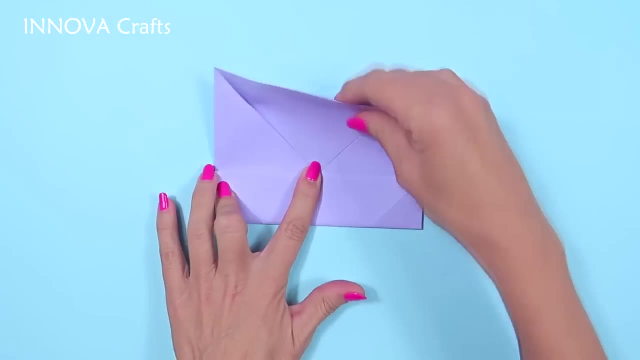 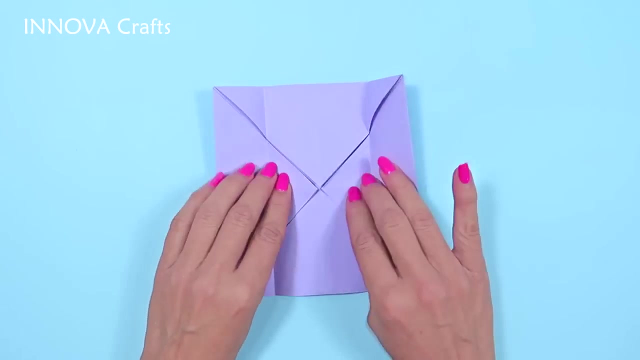 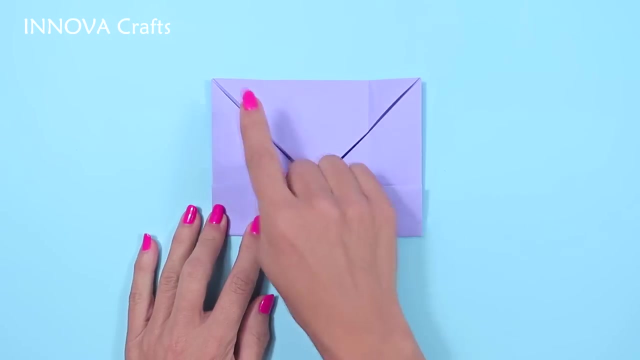 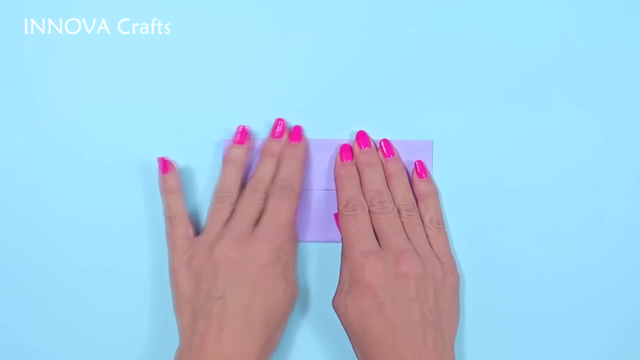 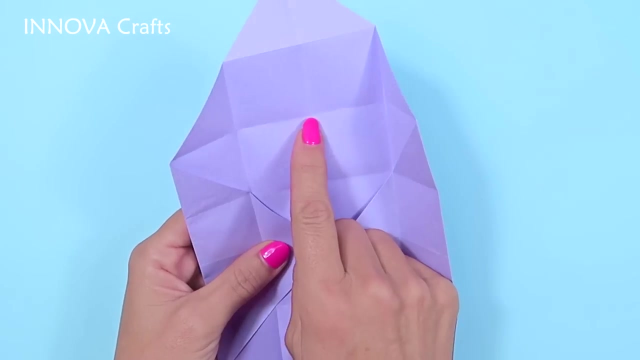 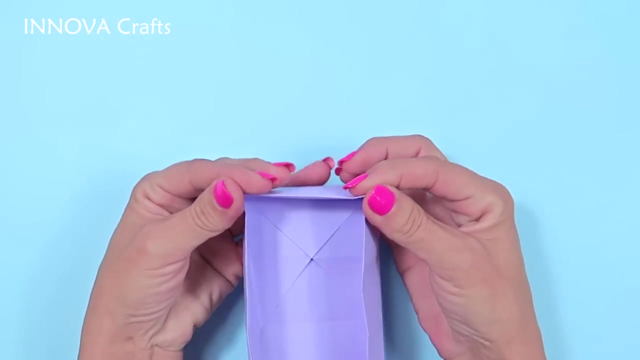 If it gets too dark? If it gets too dark, Yeah, I can carry all that you've got. Two heavy hearts is not a lot. I will put out all of the fire. We stumble and fall And it's not a lie That I die. I can't hide. 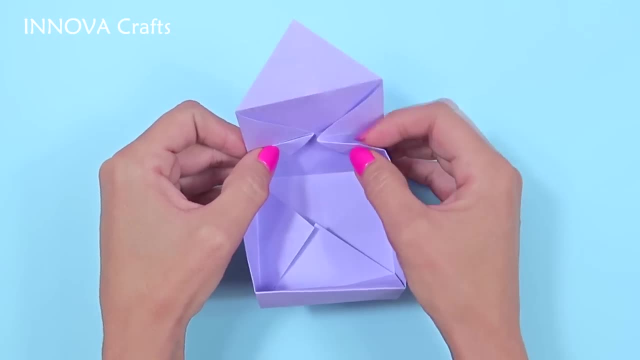 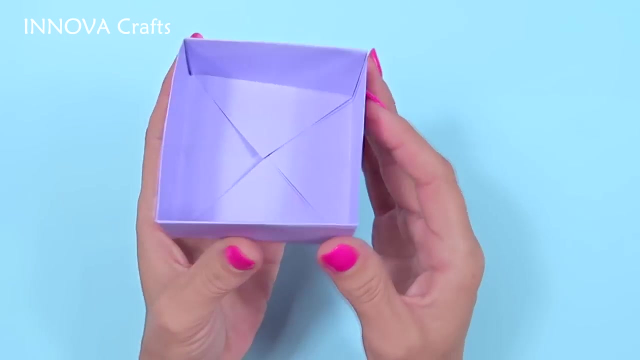 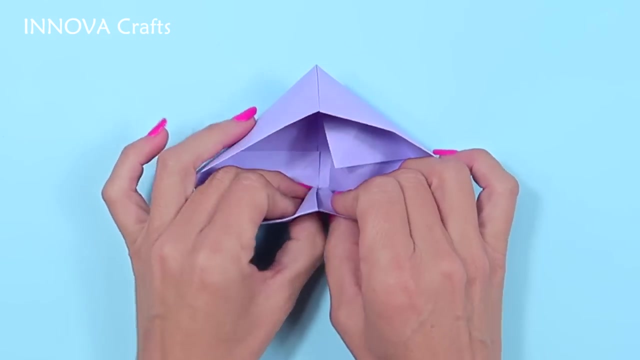 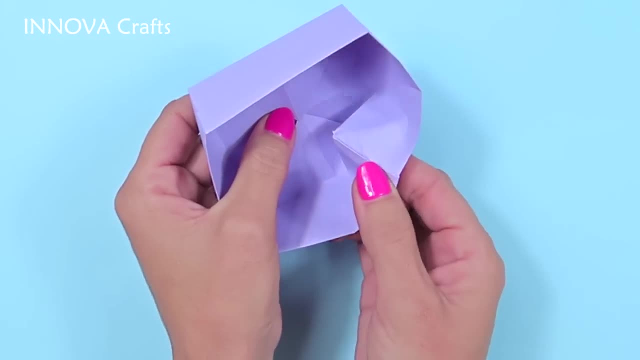 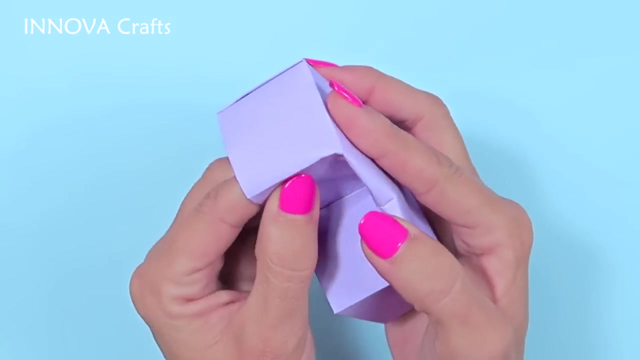 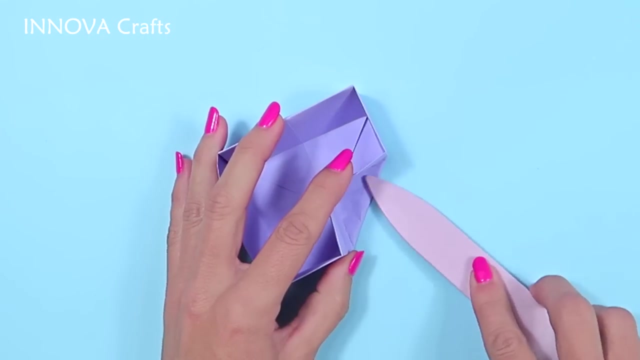 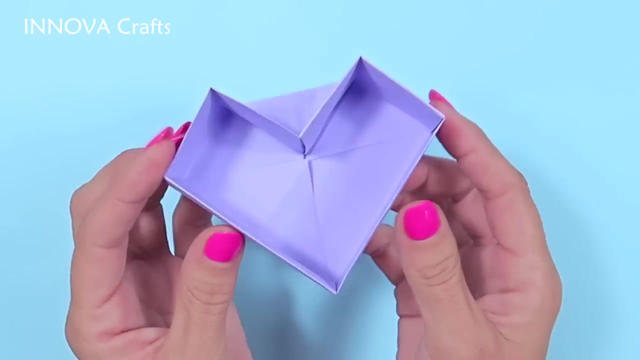 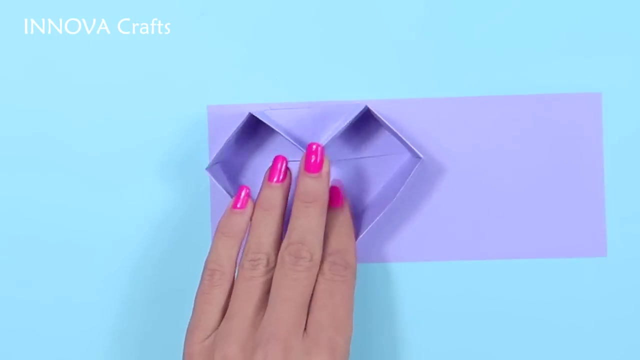 Oh, oh, I'll be your light. I'll be your light. I'll be your light. If it gets too dark, I'll be your light. I'll be your light. I'll be your light If it gets too dark. Oh, oh, I am running for you.